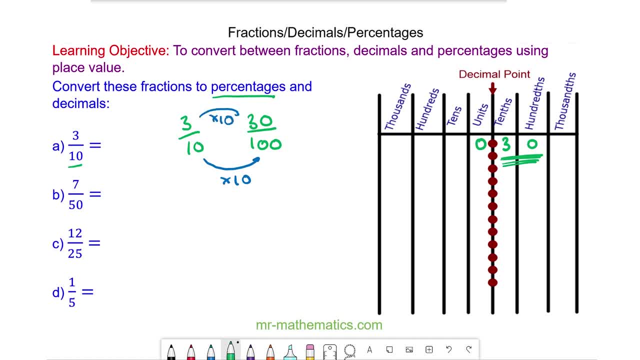 and 3 times 10 to make 30.. So three tenths is 30 percent and by writing it in a place value table you can see we've converted it to a decimal of 0.3.. The fraction: 7 over 50.. The problem we have here is that our place value table doesn't work with. 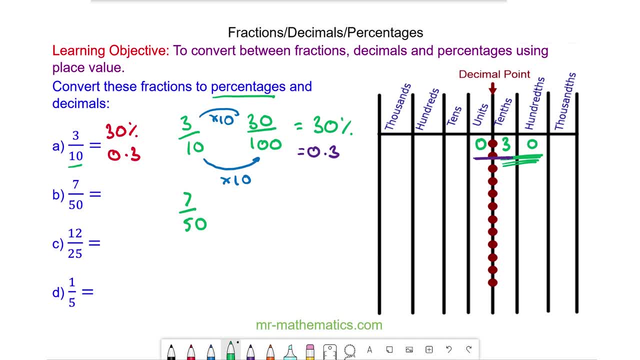 50ths, so we need to write it as a fraction which appears in our place value table, which is hundredths. So we need to write 7 50ths over 100 and to do this we can multiply the numerator and denominator by 2, because 50 times 2 makes 100.. 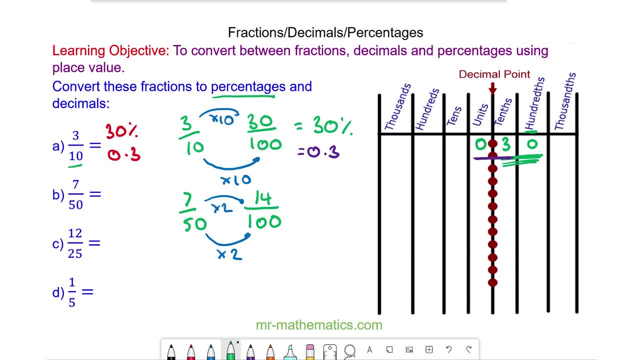 And 7 times 2 is 14.. So we have zero units, one tenth and four hundredths. So 7 50ths is 14 percent and 0.14.. Do you want to try and convert 12, 25ths and one fifth to a percentage and decimal? 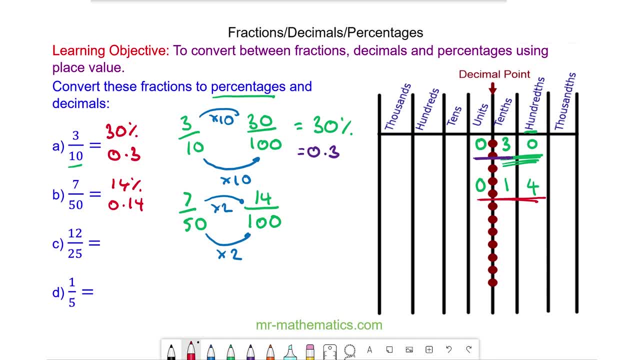 by pausing the video and you can resume it when you're ready For question c. We're going to write it as a fraction over 100.. We're doing this by multiplying the 25 by 4 and to keep its equivalent, we do the same to the 12. 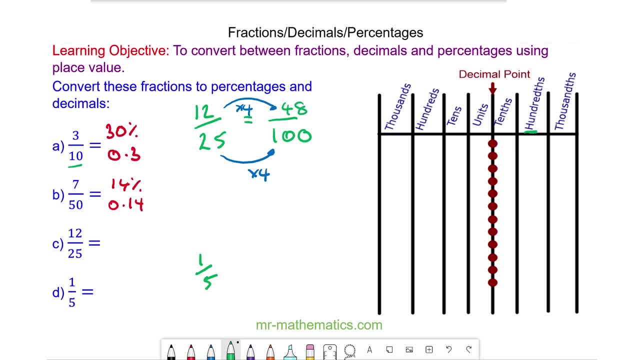 and we have 48 over the 100, which is zero units, four tenths and eight hundredths, which is 48 percent, and as a decimal, 0.4.. And the question d, one fifth, we can write as a fraction over 10., Which is 5 times 2, and 1 times 2, which is 2 tenths. 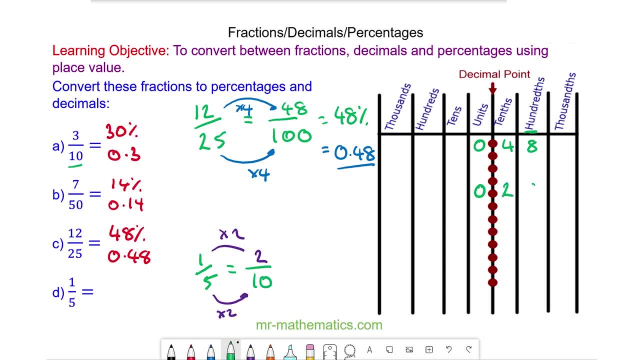 So we have zero units, two tenths and zero hundredths, which, as a percentage, is 20 over 100.. Another decimal: 0.4.. And the next question, d. We can write it as a fraction over 10, which is 5 times 2, and 1 times 2, which is two tenths. so we have zero units, two tenths and zero hundredths, which, as a percentage, is 20 over 100.. 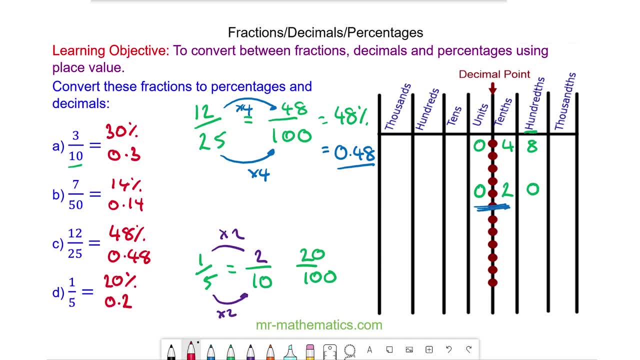 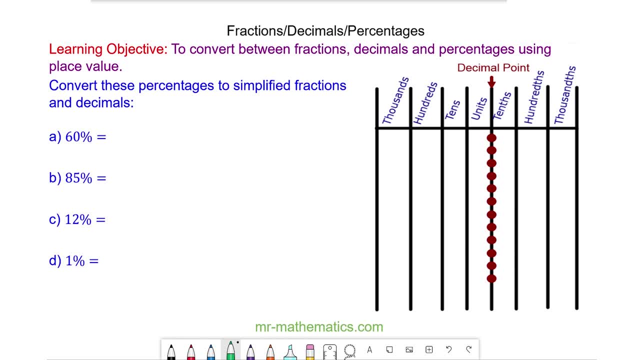 0.2.. Okay, let's try some more questions. So now we're going to convert these percentages to simplified fractions and decimals. We begin with 60%. We know percentage means a fraction of 100.. So we have 60 over 100, which is 60 hundredths and no units. So we know at a decimal. 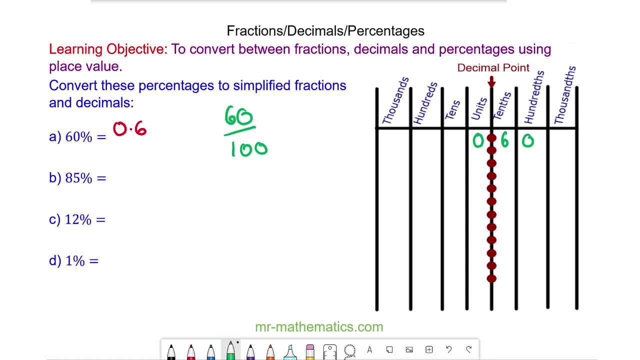 it is 0.6.. And we can simplify this fraction by dividing both by 10, because 10 is a factor of 60 and 100. So we have 6 over 10.. And we can simplify it further by dividing both by. 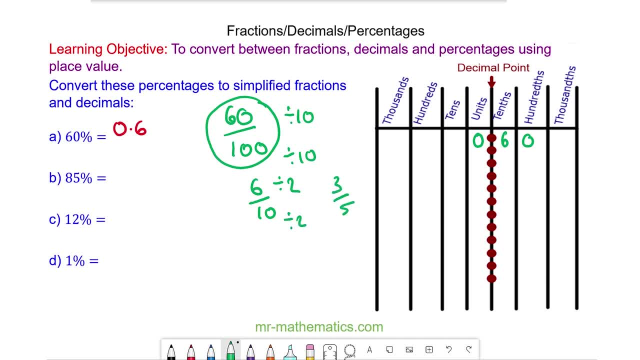 2. So we have three fifths For 85%, we have 85 over 100, which is zero units, eight tenths and 500.. So not 0.85.. And as a simplified fraction, we can divide the numerator and denominator. 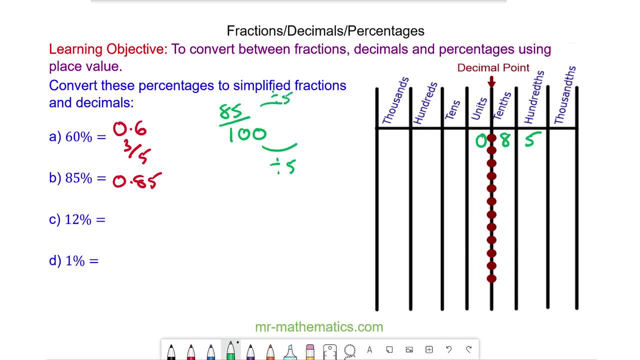 by five. 85 divided by five is 17.. 100 divided by five is 20.. And this is our simplified fraction. Do you want to try and convert 12% and 1% to a simplified fraction and decimal By pausing the video and you can resume it when you're ready? 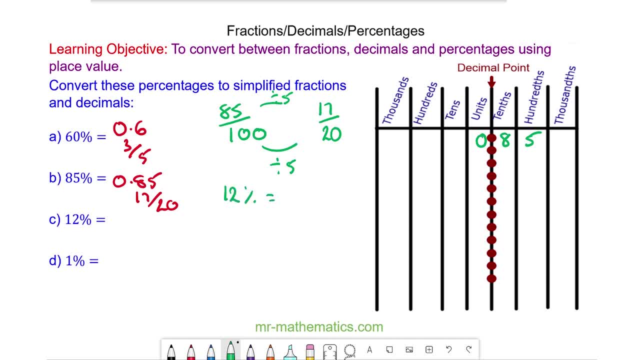 For question C: 12%, we know, is 12 over 100, which is zero units. one tenth and two hundredths, So not 0.12.. And we can simplify the fraction by dividing both by two, So we have six fiftieths. 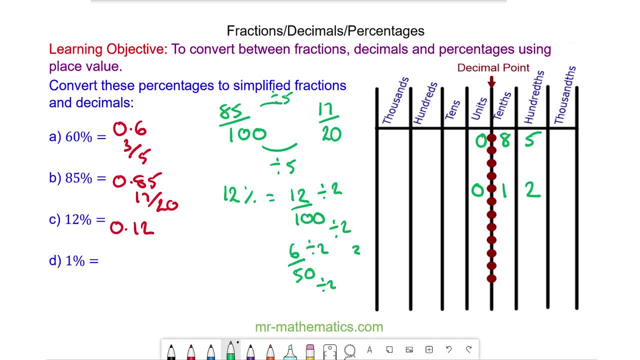 We can divide by two again. So we have three, twenty, fifths. And finally, for question C, we know is 12 over 100, which is zero units, one tenth and two hundredths, And we can simplify the fraction by dividing both by two. So we have six, fiftieths. We can divide by two again. 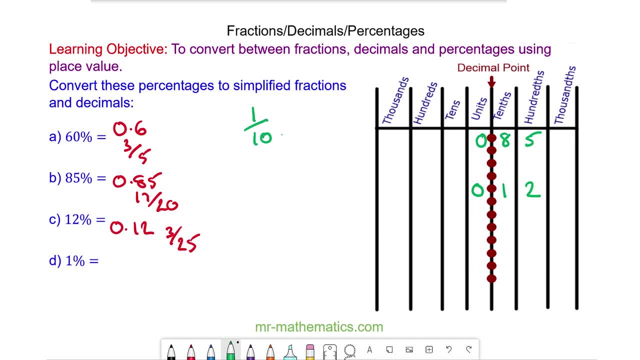 For question D: 1% is one over 100, which is no units, no tenths, one hundredth as a decimal, not a point zero one, And it cannot be simplified any further. So again, one over 100. 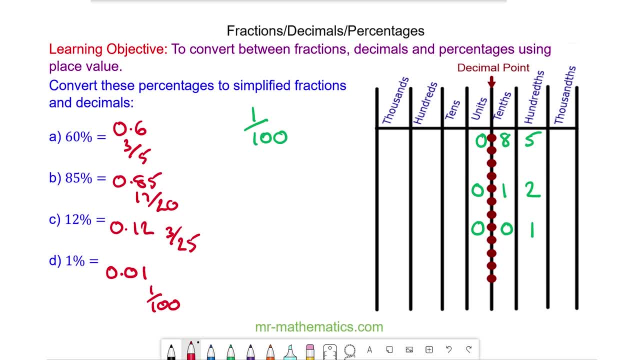 Okay, thank you for watching and I hope you found that useful. Thanks again and take care. Bye-bye.